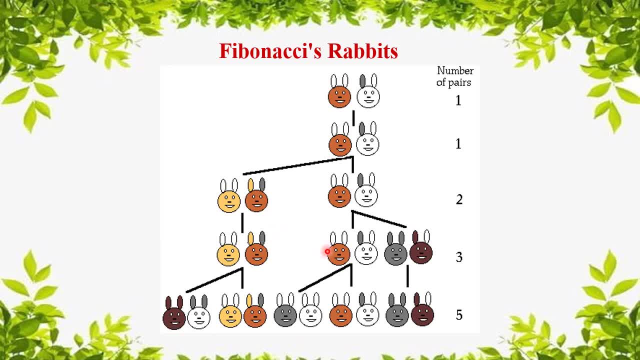 rabbits in the field. At the end of the third month, the original female produces a second pair, making three pairs in the field, all in the field. at the end of the fourth month, the original female has produced it, another new pair. the female born two months ago produces her first pair, also making five pairs. so we get the. 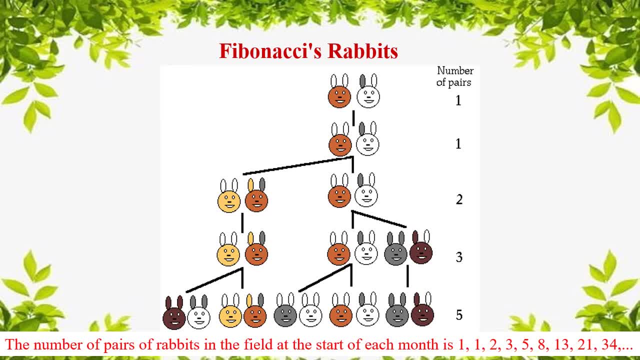 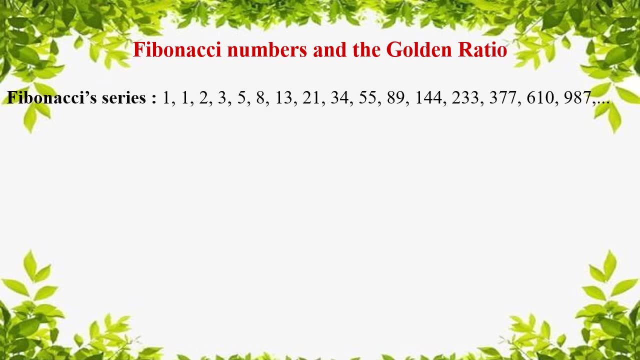 number of pairs of rabbits in the field at the start of each month is 1. 1, 2, 3, 5, 8, 13, 21, 34, like this. so we can easily say that each number in the fibonacci series is the sum of the preceding two. 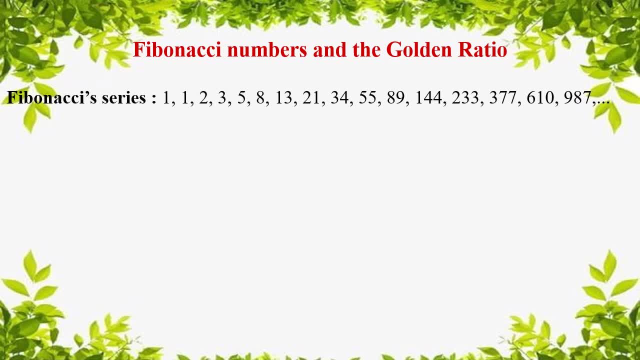 numbers. next we are going to see what is golden ratio. if we take the ratio of two successive numbers in fibonacci series and we divide each by the number before it, we will find the following series of numbers like: second number in the series is 1. first number is 1. 1 divided by 1 equal to 1. 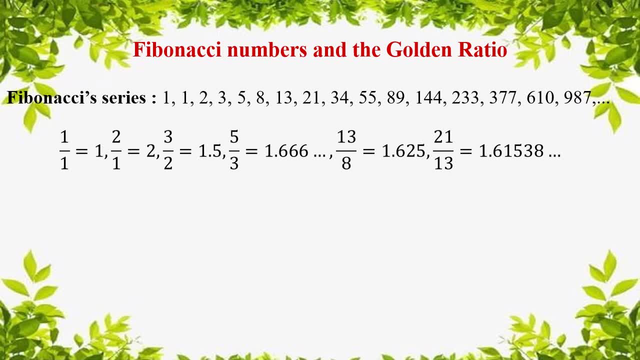 third number is 2. second number is 1: 1. 2 divided by 1, equal to 2. fourth number is 3. third number is 2, so 3 divided by 2, equal to 1.5. like this it goes on. the important thing we are noticing here is: after fourth ratio, all. 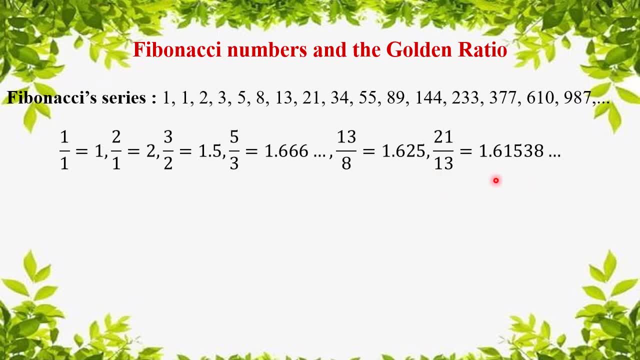 the numbers are seem similar, so it is easier to see what is happening. if we plot the ratios on a graph, the numerator numbers are taken as i in the x-axis, the answers, which means the ratios, are taken as five in the y-axis. so if we plot the coordinates, 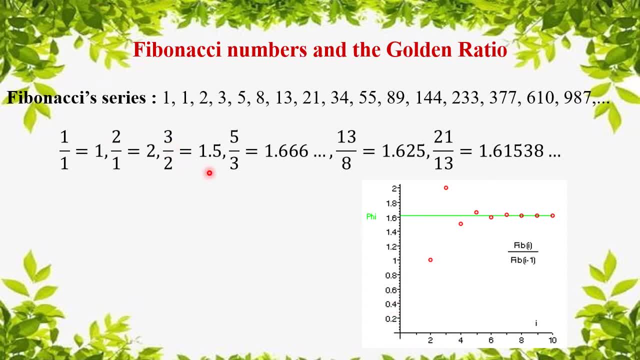 like 1 comma 1, 2 comma 2, 3 comma 1.5, 5 comma 1.6, 7, 13 comma 1.625, 21 comma 1.615. so this graphs is like that the ratio seems to be settling down to 1.625 and the ratio seems to be settling down to. 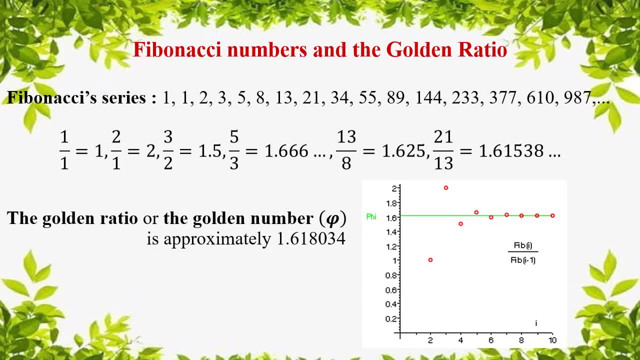 a particular value, which we call the golden ratio or the golden number. it has a value of approximately 1.618034. the golden ratio 1.618034 is also called a golden section, or the golden mean, or just the golden number. it is often represented by a greek letter, phi, so phi is approximately 1.618034. 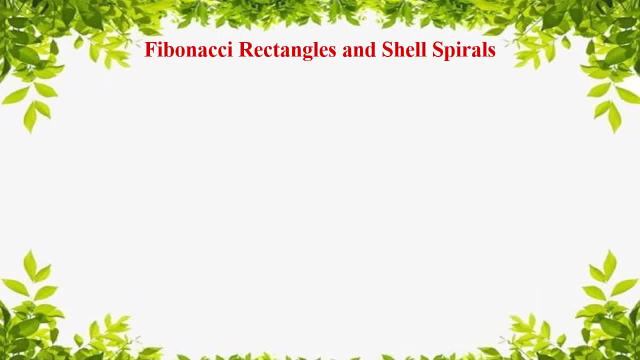 the golden ratio or the golden number, it has a value of approximately 1.618034. next, we define the function of this sequence. like we know, nth term is the sum of two preceding terms, that is, n minus 1th term and n minus 2th term. 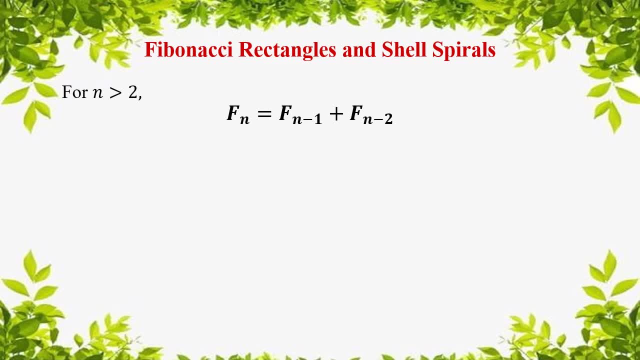 for n greater than 2 fn equal to fn minus 1 plus fn minus 2. so this function gives us the following sequence: this is called fibonacci sequence: 1, 1, 2, 3, 5, 8, 13, 21, etc. we can make another. 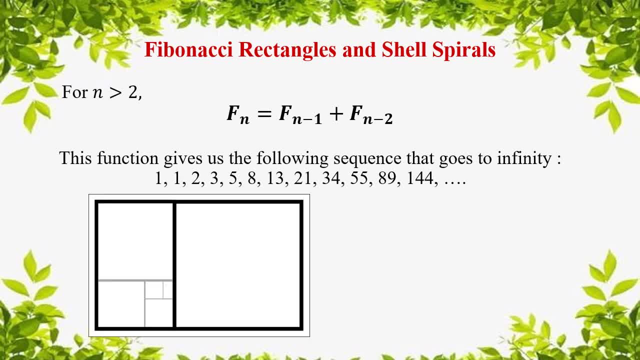 sequence which is showing the fibonacci numbers. if we start with two small squares of size 1 next to each other, in the below of both of these squares draw a square of size 2, that is 1 plus 1. we can now draw a new square touching both a unit square and the latest square of size 2. 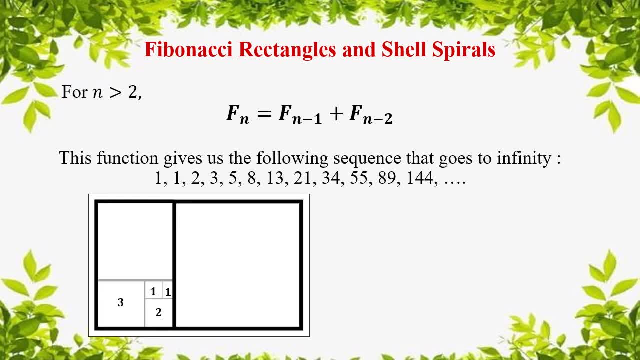 so having sides three units long and then another touching both the two square and the three square, which has the size of five units. we can continue adding squares around the picture, each new square having a side which is as long as the sum of the latest two squares sides. 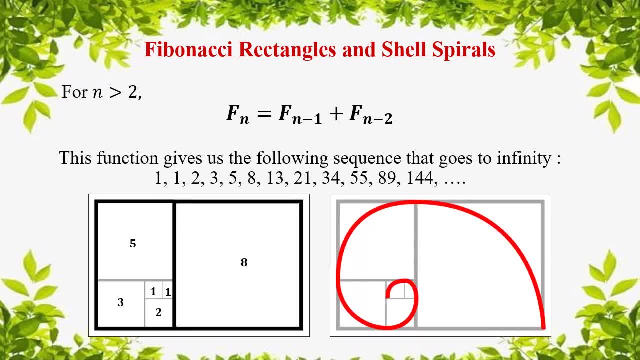 this set of rectangles are called fibonacci rectangles. here is a spiral drawn in the squares, a quarter of a circle in each square. such spirals are seen in the shape of shells, of snails and sea shells and, as we see later, in the arrangement of seats. on flooring plants too. the spiral in the squares makes a line from: 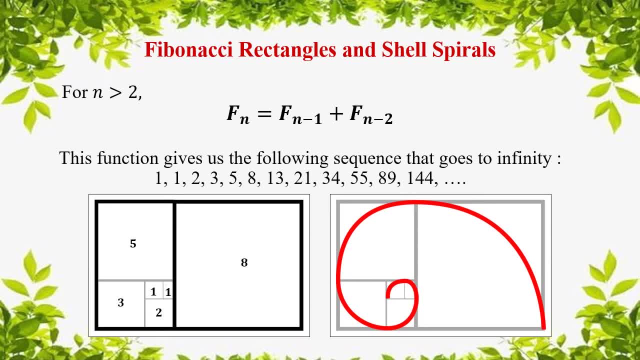 the center of the spiral, increased by a factor of the golden number in each square. so points on the spiral are 1.618 times as far from the center. after a quarter, turn in a whole. turn the points on your radius out from the center or 1.618 whole power 4, that is 6.854. 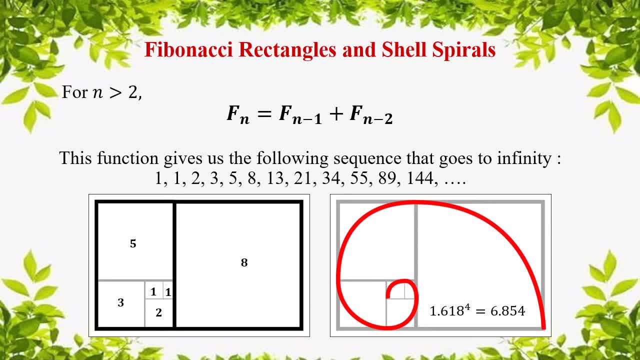 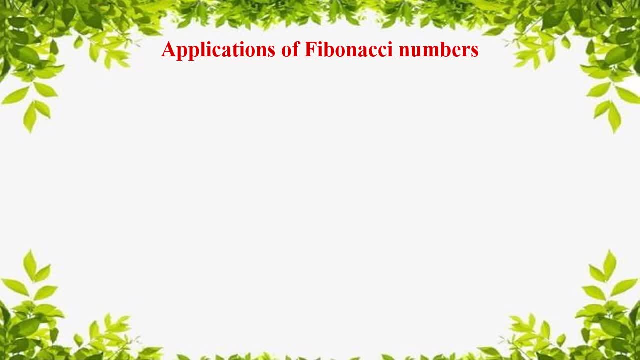 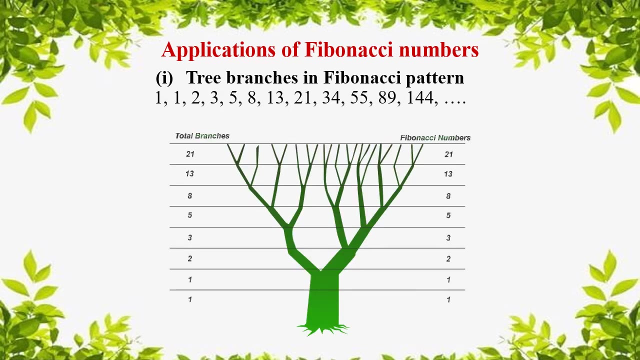 so this is a whole concept of fibonacci rectangles and shell spirals. so in the second part we are going to see some interesting applications in fibonacci numbers and golden ratios. it will be mind-blowing things, uh. first one is tree branches in fibonacci pattern. so plant in particular shows the fibonacci numbers in the number of growing points that it has. 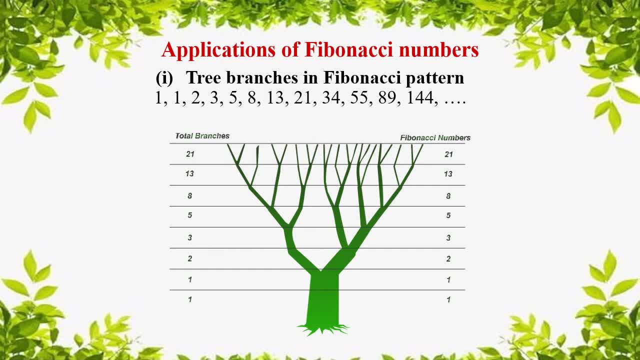 suppose that when a plant puts out a new shoot, that shoot has to grow two months before it is strong enough to support branching. if it branches every month after that, at the growing point we get the picture shown here. a plant that grows very much like this is a sneeze word. 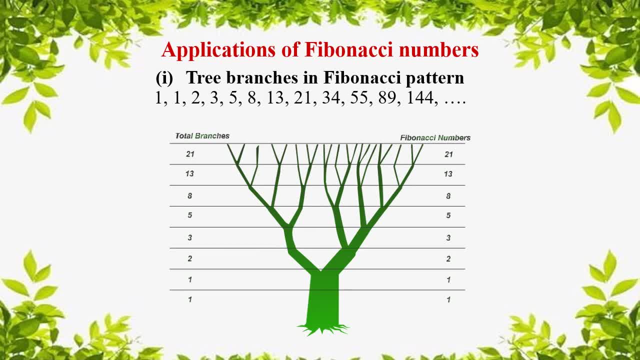 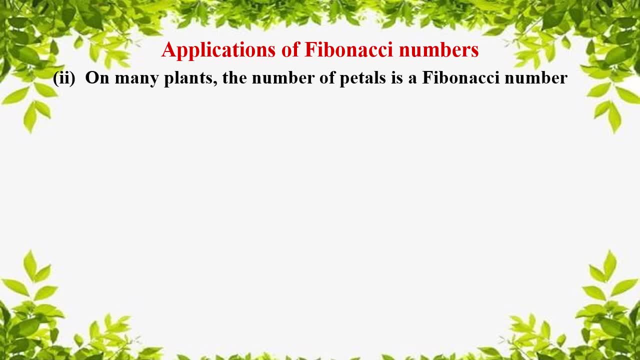 So this is an example of this pattern. So second example is: on many plants the number of petals is a Fibonacci number. For example, buttercups have 5 petals, lilies and iris have 3 petals and some flowers have 8,, 13,, 21,, 34,, 55,, 89. like this Fibonacci numbers. 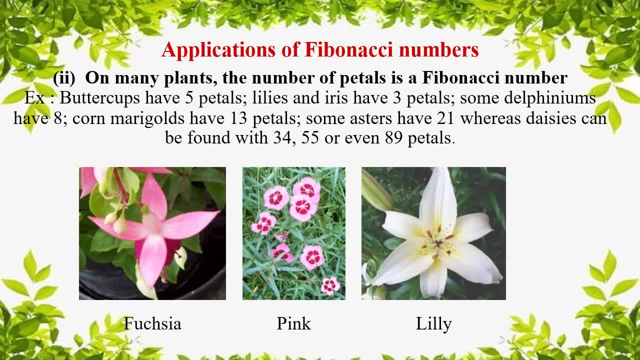 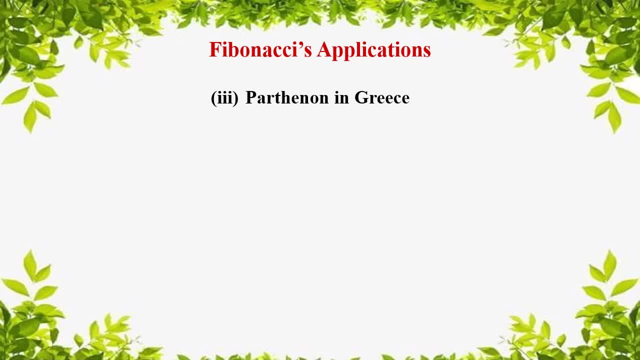 But very few plants show 4 petals like. 4 is not a Fibonacci number, So third beautiful example is Parthenon in Greece. As we know earlier, many buildings and artworks have the golden ratio in them. An example would be the Parthenon in Greece. 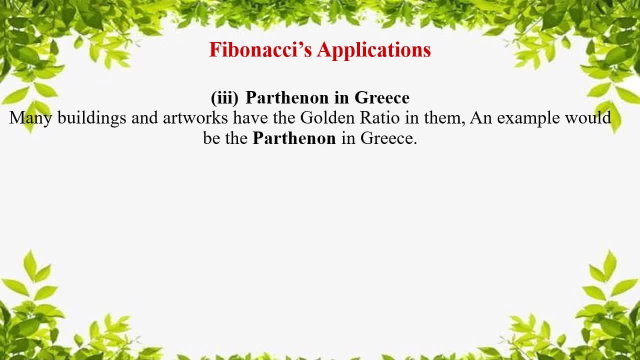 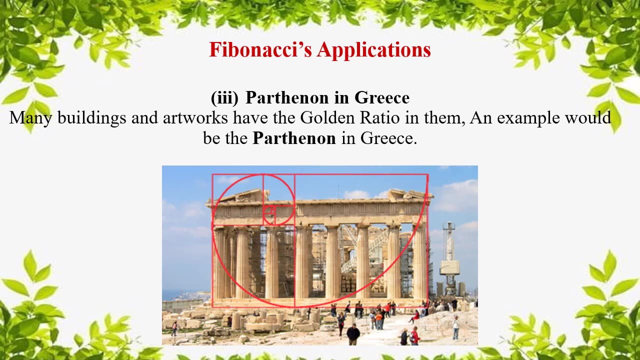 Golden spiral supremo shanti Parthenon building in Greece, but there is no evidence that the golden ratio played a role in the design of this building. It is present in geometry. Here we can see the image of this spiral: supremo shanti Parthenon in Greece. 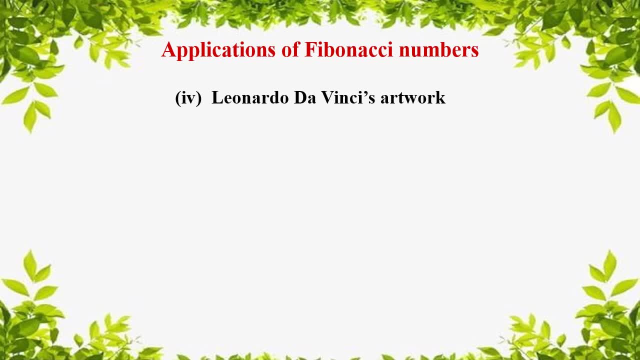 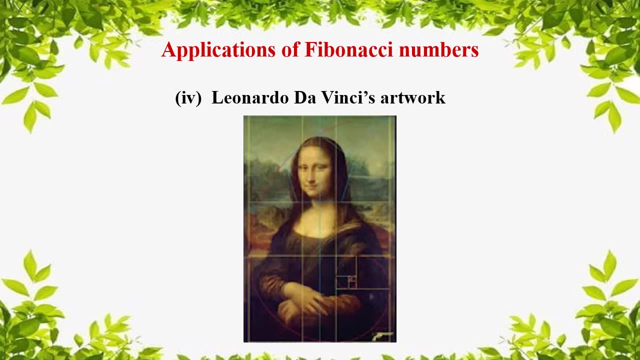 Fourth one is Leonardo da Vinci's artwork. One very famous piece known as Mona Lisa, painted by Leonardo da Vinci, is drawn according to the golden ratio. Actually, the golden proportion can be found throughout the human body. The Mona Lisa has many golden rectangles Through the painting. by drawing a rectangle around her face, we can see that it is indeed golden. if we divide that rectangle with a line drawn across her eyes, we get another golden rectangle, meaning that the proportion of her head length to her eyes is golden. there are other golden rectangles that can be drawn on the rest of her body, like from her neck to the top of her hands. 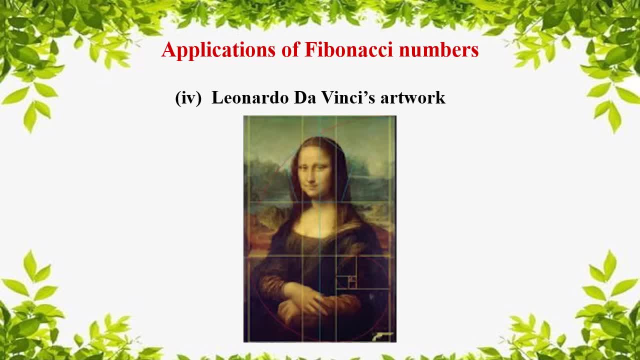 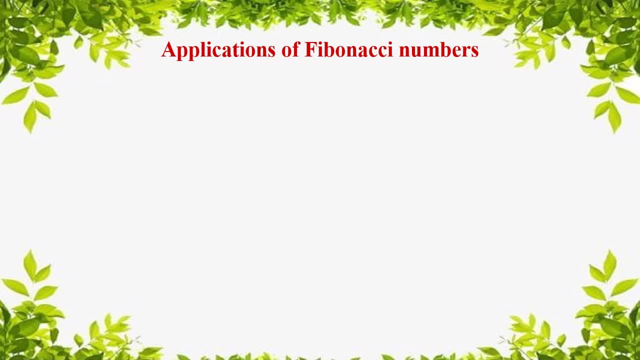 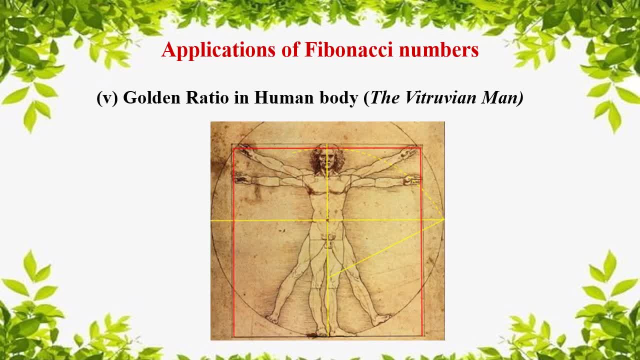 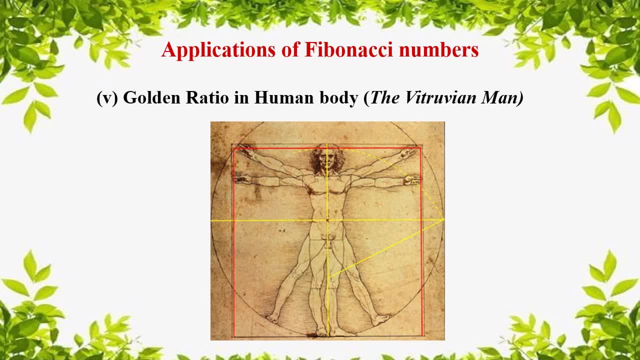 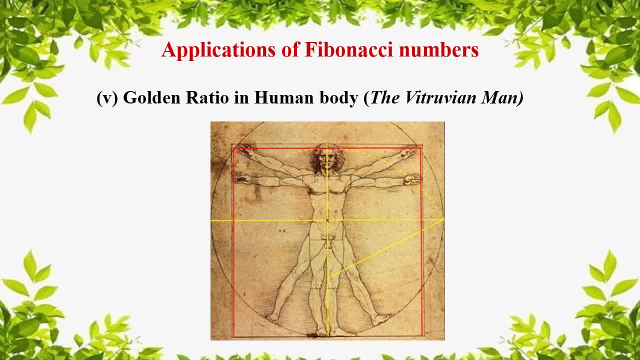 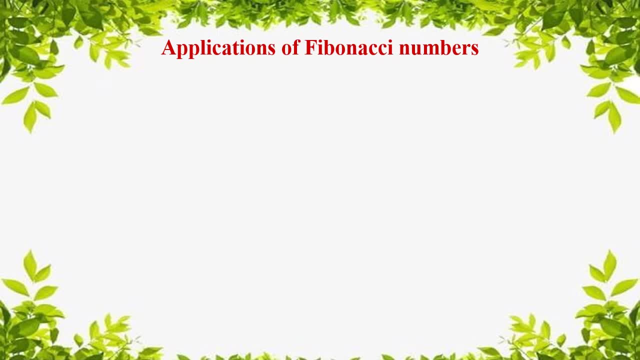 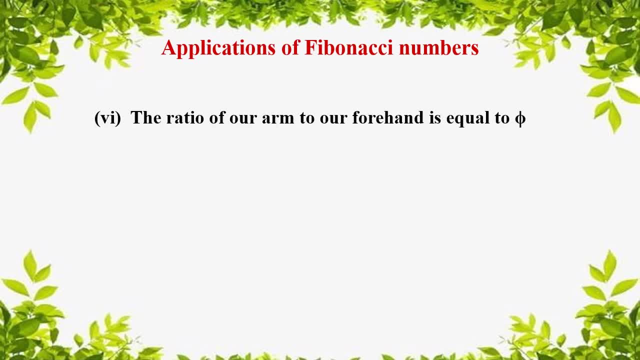 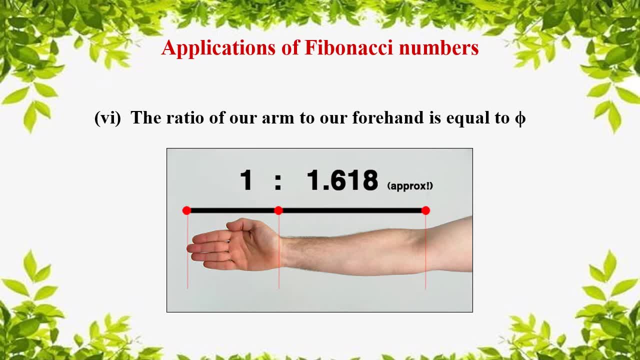 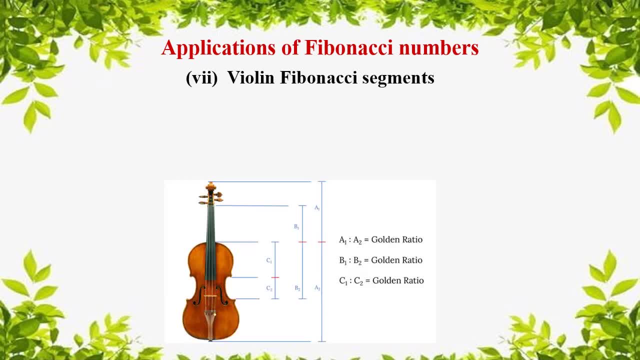 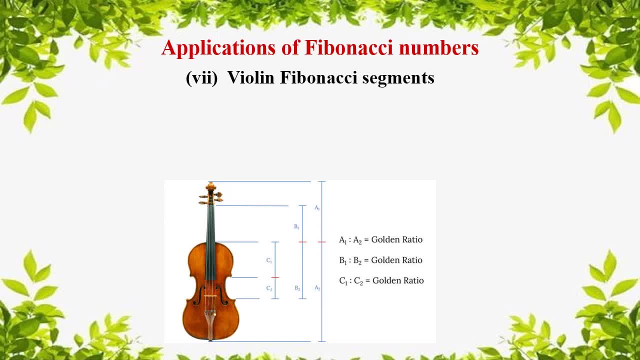 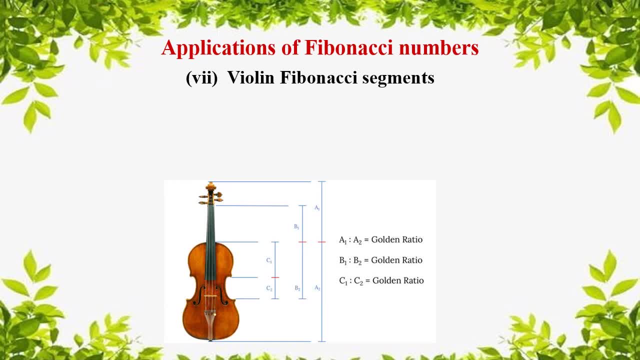 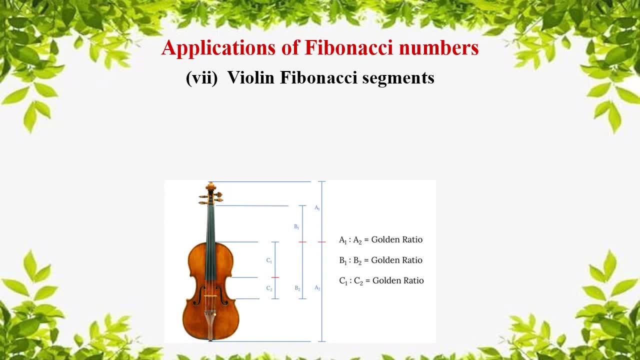 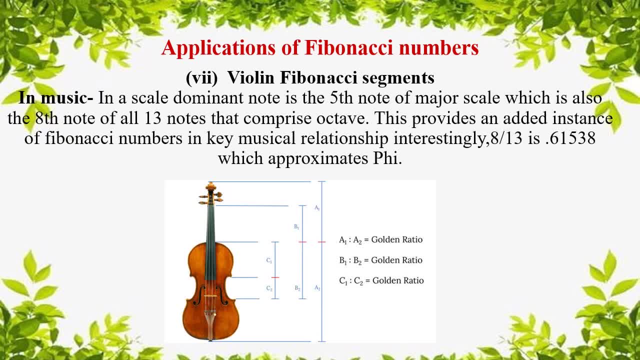 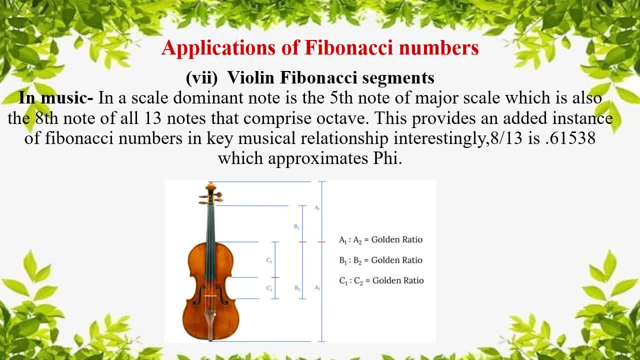 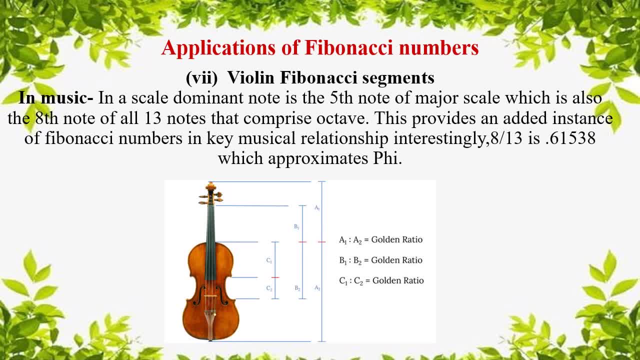 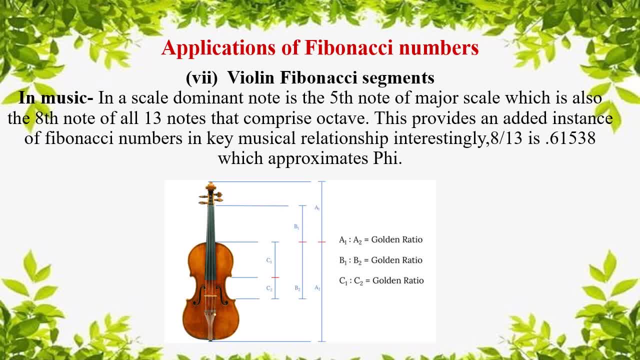 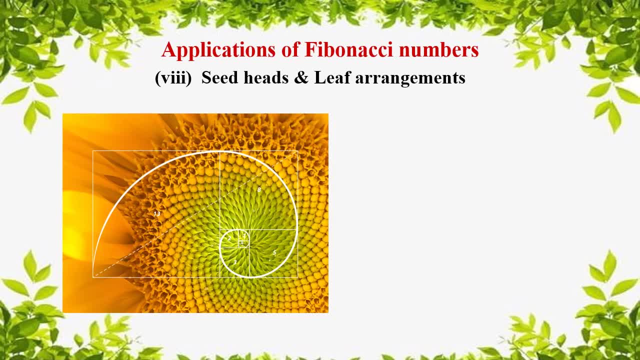 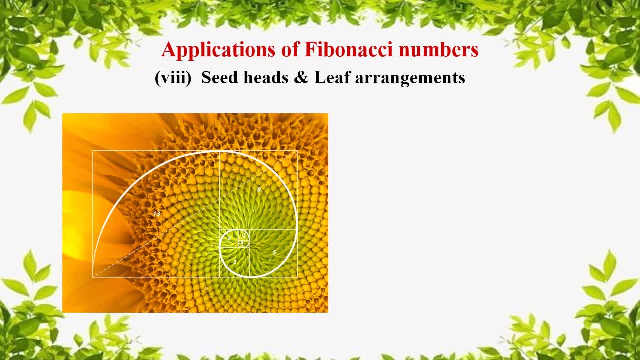 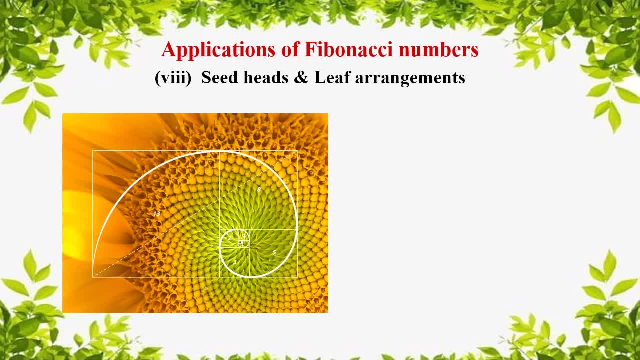 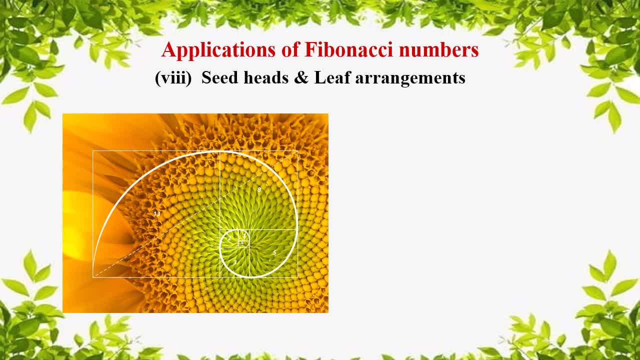 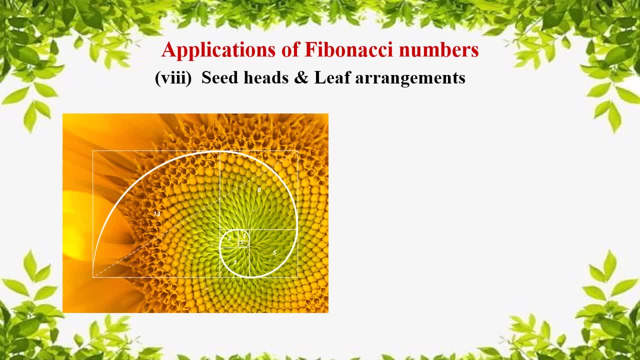 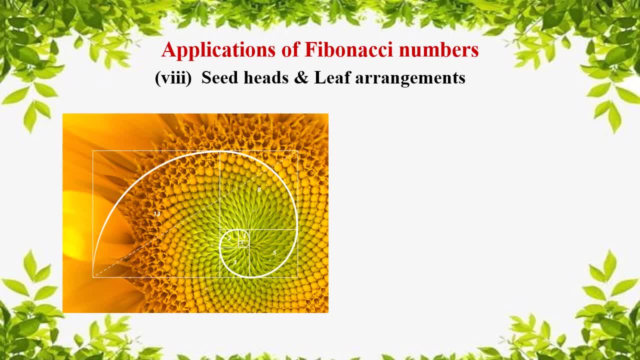 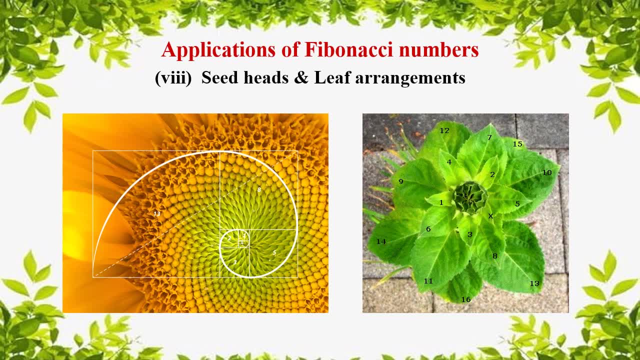 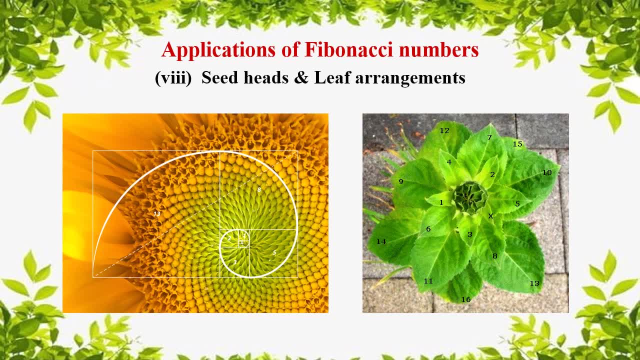 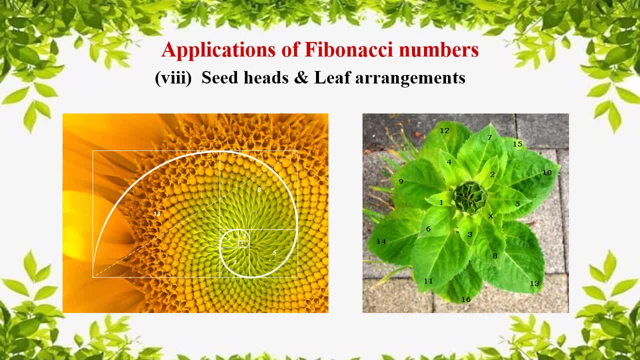 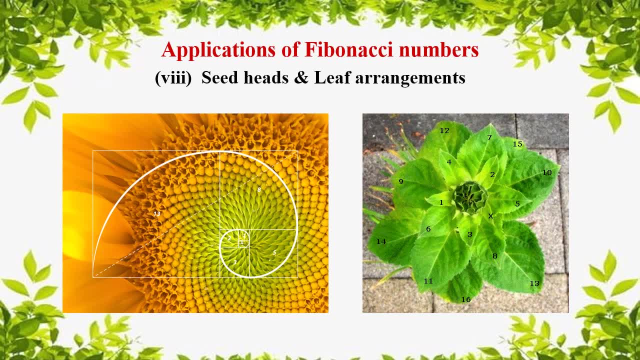 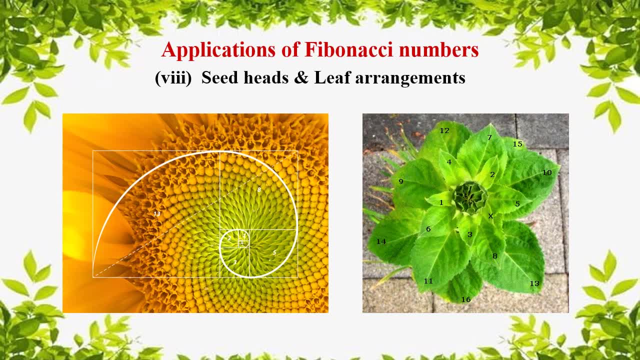 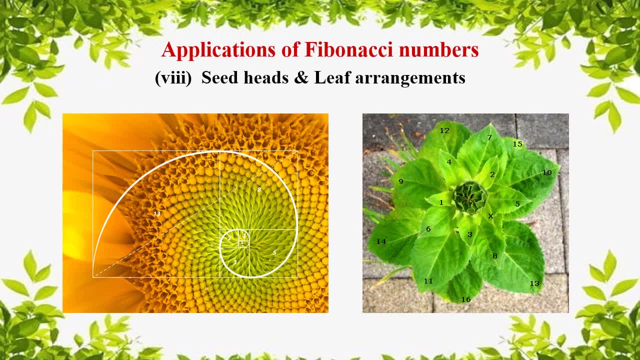 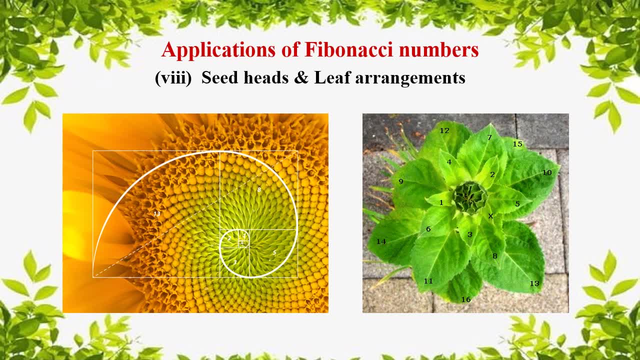 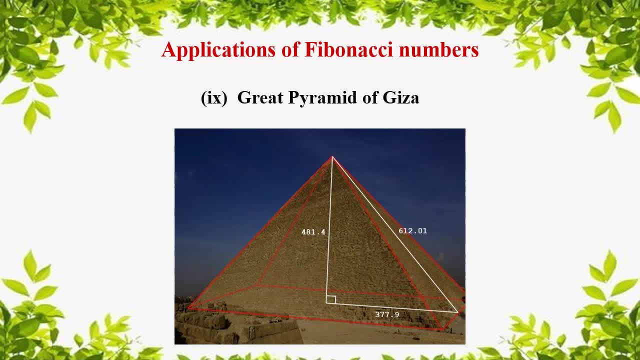 The Last Supper Old Man and The Vitruvian Man, Giza. So this shows golden ratio concept. The height of this premier is 481.4 meters and base is 377.9 meters. So if you make this as right angled triangle by Pythagoras theorem, the 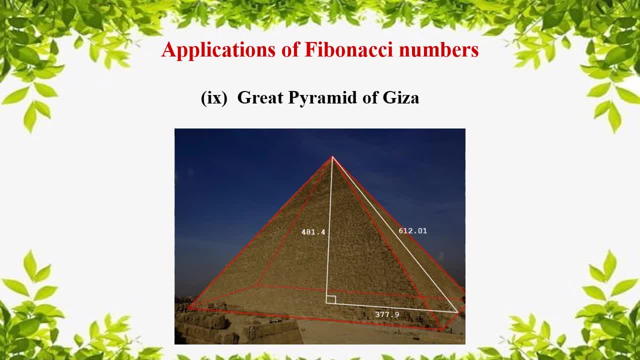 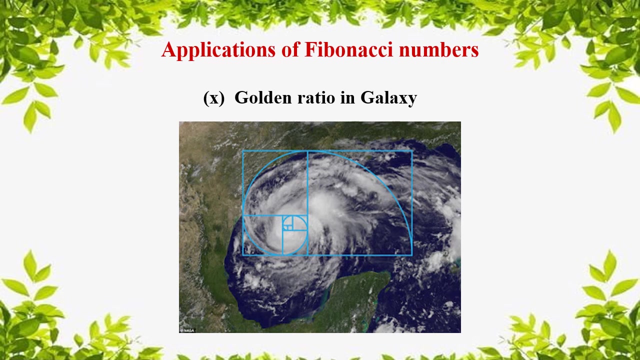 hypotenuse will be 612.01 meters. We can calculate this by using Pythagoras theorem. When we divide hypotenuse by base, we get golden ratio approximately 1.61950.. So 10th example is golden ratio in galaxy. Our galaxy clearly shows how golden ratio forms by golden triangles. 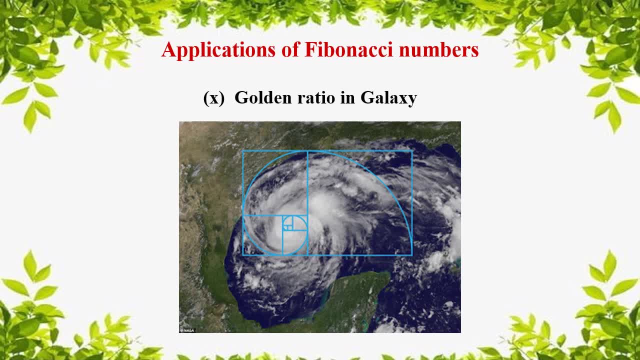 as we can see this image. So the last example is logos. So our logos is in the golden triangle. So we can see this image. So the last example is logos. So our logos is in the golden triangle. So the last example is logos. So our logos is. 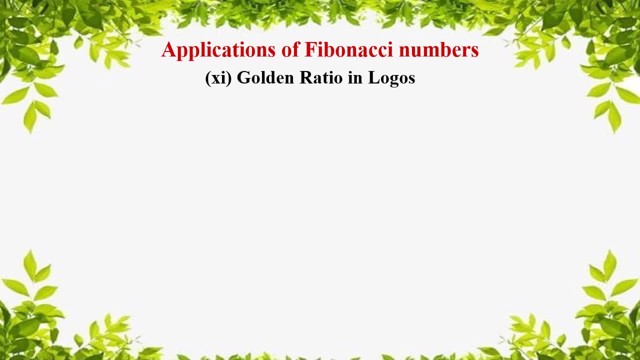 in the golden ratio. The famous logos in our daily product, like Twitter, Apple, Pepsi and many more applications, have the logos by using of golden ratio. So, finally, I would like to tell you that the golden ratio related not only to aspects of mathematics, but also to 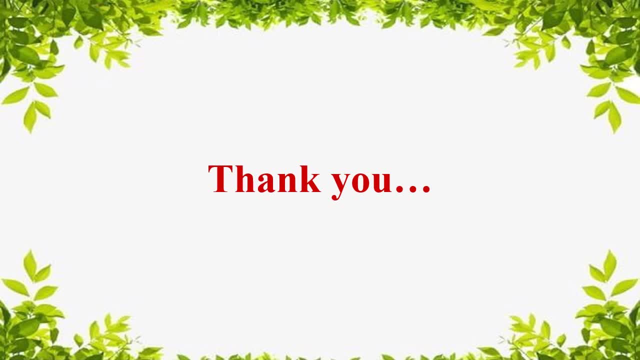 physics, chemistry, biology and the topology of space time. So make use of this video to understand how deep our life is related to mathematics. Thank you.